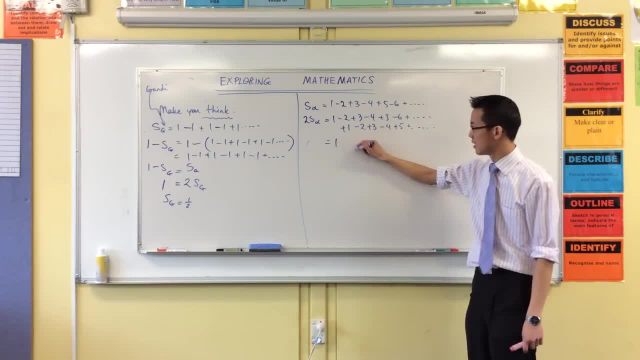 term, with the second term, with the first term, What do you get? You get minus 2 plus 1, which is minus 1.. Right, Yeah, Plus 3 minus 2.. That's plus 1.. Minus 1.. Plus 1.. Minus, Okay, hold. 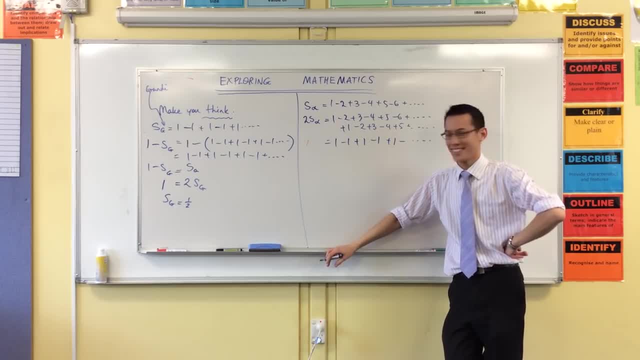 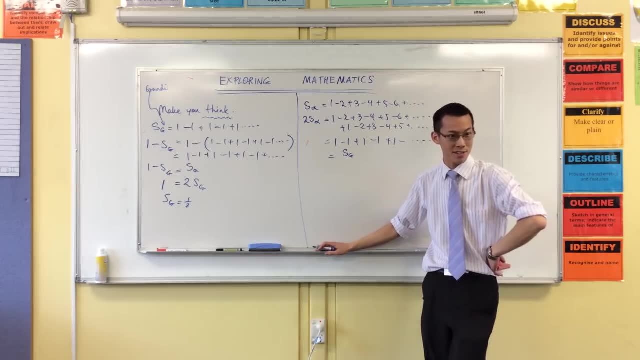 on. I recognize this guy too. Right, That's the series I started with. But I also know what that series is equal to. That's a half, isn't it? Allegedly that's a half, That's a half, Okay. So if I want to know what the actual series is, I'll divide again. No. 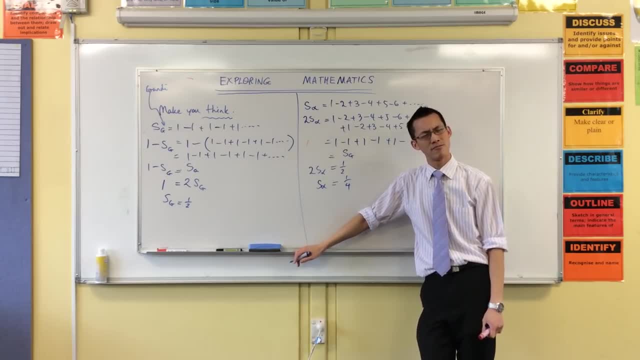 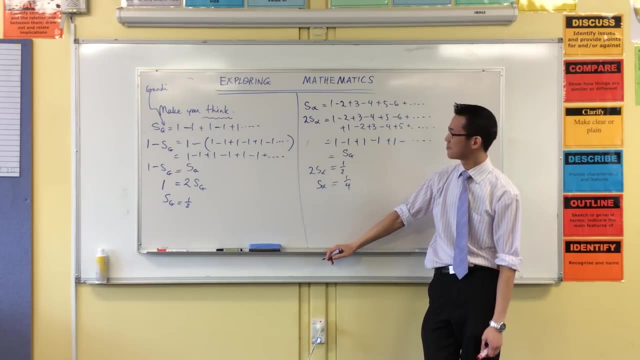 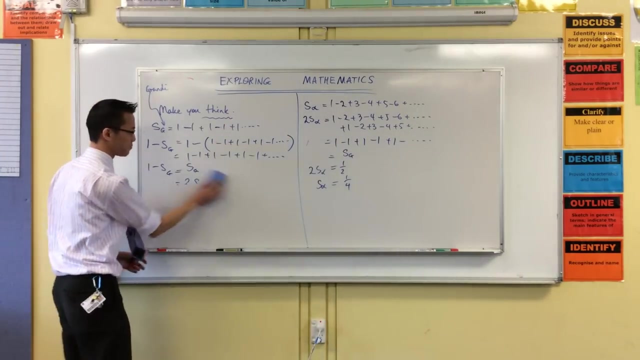 problems. That's a quarter. Really, Have I made you think yet? Okay, hold on to your hats, because here's the last step. Here's the last step and I'm really going to bend your brain. Okay, There are three stages here. Three stages. 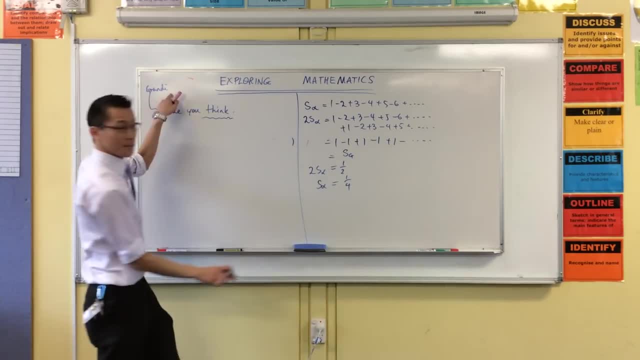 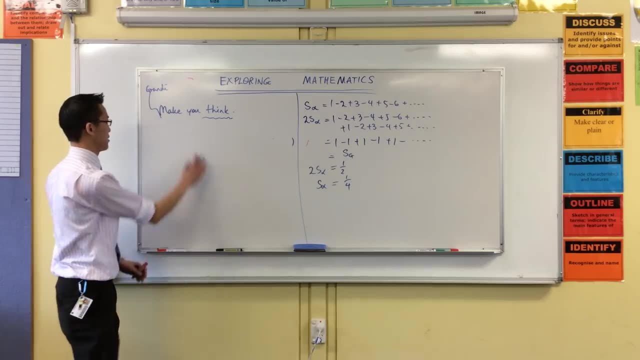 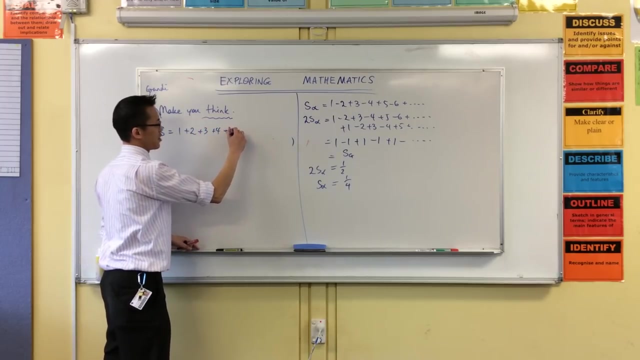 Okay, First step was that Grandi series, This guy- Okay, Second step was this related series which you can see has a relationship. Okay, Here's the last series. I'm just going to call it S Okay, And it doesn't look well. it looks pretty ordinary compared to the other. 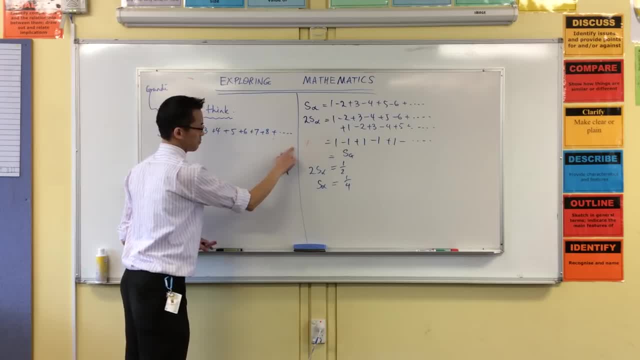 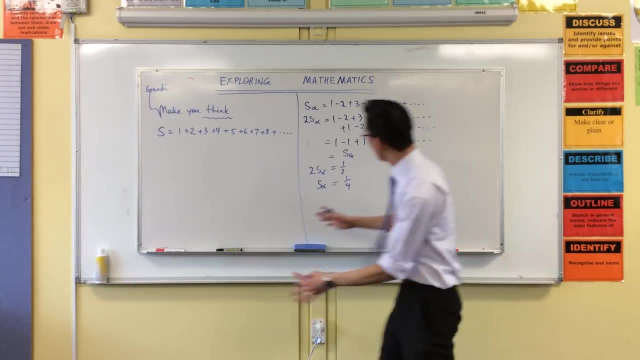 ones, right, Looks decidedly ordinary. Okay, Now, by the way, by the way, the series I started with and then the series I started with, I'm going to call it S. Okay, So I'm going to call it S. So, what people we started with and then this series, right, they had. 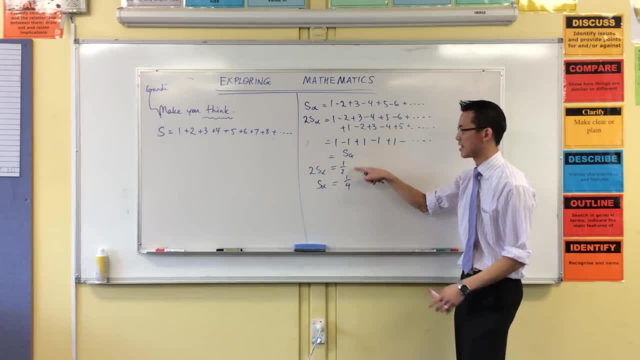 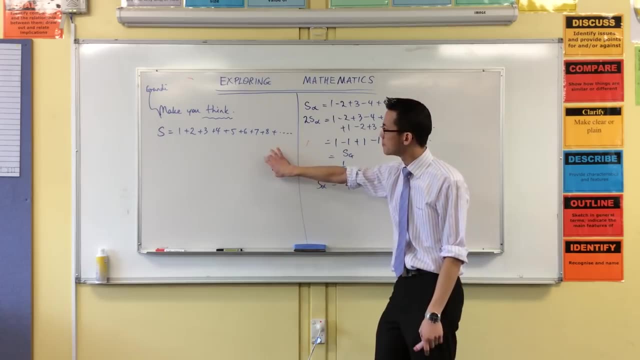 some alternating business happening right, And so that's kind of what. let us get a value at the end. Do you think we can get a value for this? Hmm, now I'm going to do this again On the count of three. okay, I want you to look at this and I want you to settle. 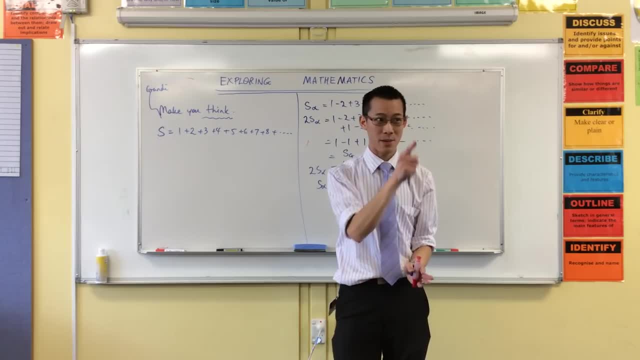 in your mind It could be wrong. It's fine. Mathematicians are wrong all the time. That's why they discovered cool stuff. okay, But I want you to see what you would say. What do you think this whole thing would be if it was right? Tell me, Oh, okay, So I'm going. 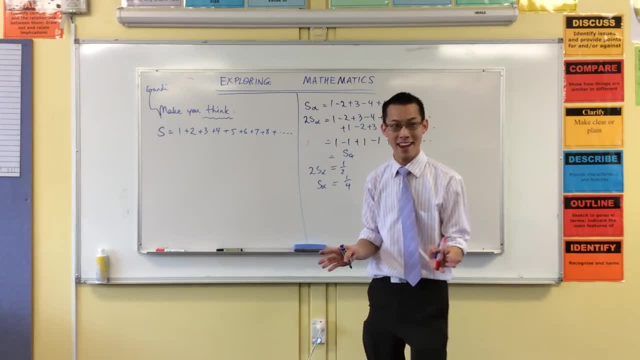 to do this again. I want this to look at this way, So I'm going to settle in your mind: It's equal to on the count of three. I'm going to ask you all to say it once. Okay, you ready, Okay. 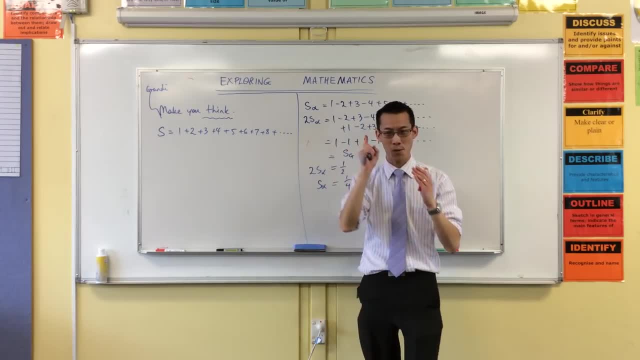 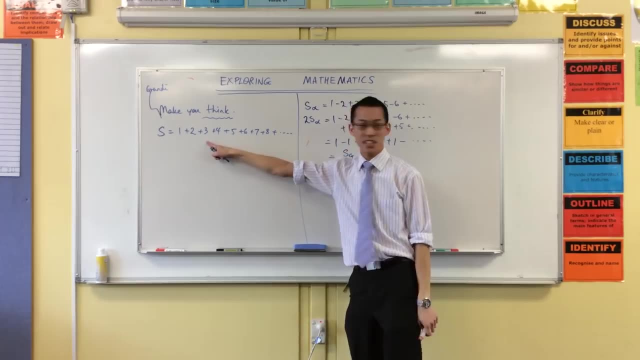 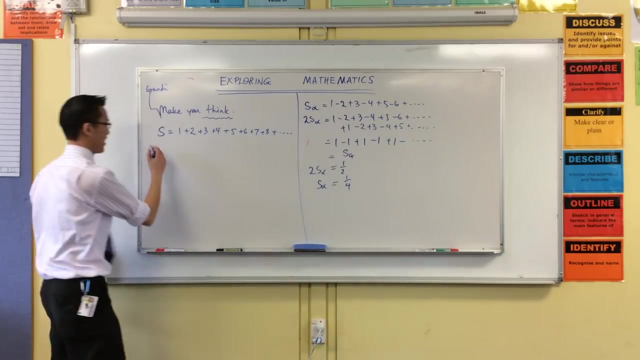 Think about it In your head. Count of three: One, two, three. Not a bad guess. Not a bad guess Because it's going to keep on growing forever, Right? Guess what? I've got news for you. The question is: how will I? 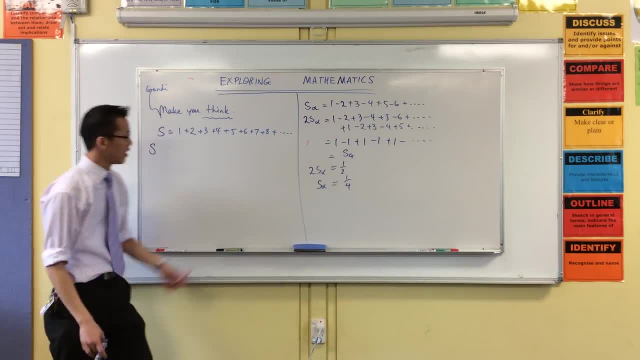 show you. Well, I laboured all these points to show all of this. I'm going to take this sum and, if I've got it right, I am going to subtract this alpha series. This guy, I'm going to take him away. 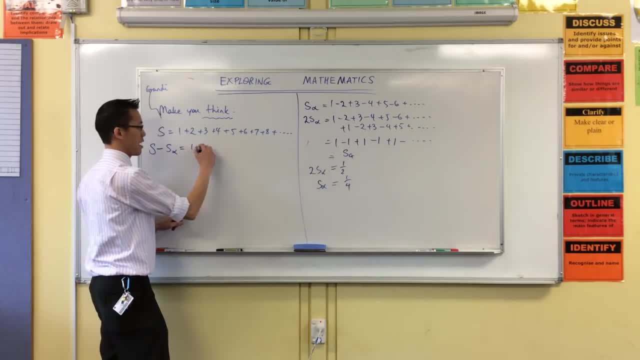 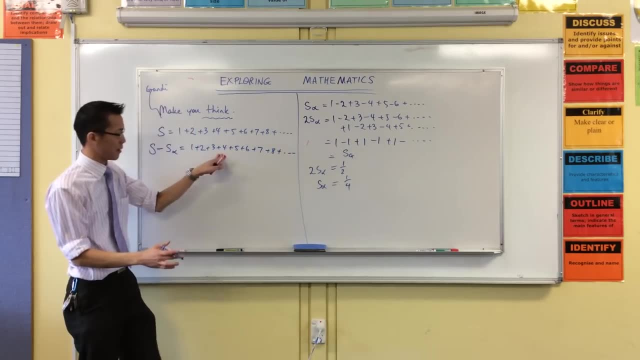 So, again, I'm going to write this very carefully. Here's my original one. This is the sum of all the counting numbers And, by the way, it's actually important that you write quite a few of them, So don't just stop at three or four. 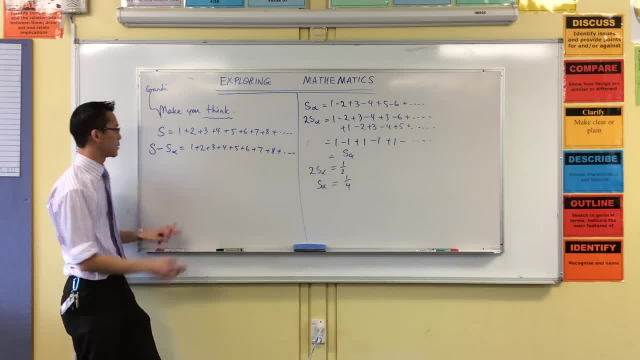 Write a few of them out- Eight at least, I think. Now I'm going to subtract this series in here. I'm going to write it directly beneath- Okay, I need to rub that up properly Subtract. And this series looks like this: 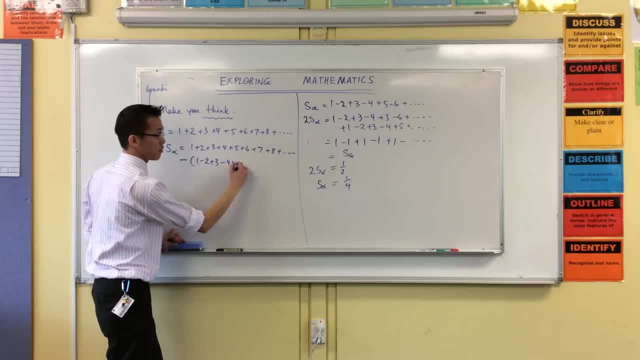 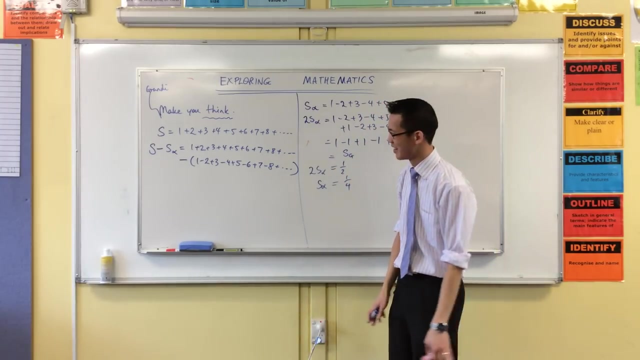 One minus two plus three minus four plus five minus six plus seven minus eight, and so on. Okay, Now, just like before, we have some brackets to deal with. Right, But we can deal with brackets, No problems. There's a minus sign. 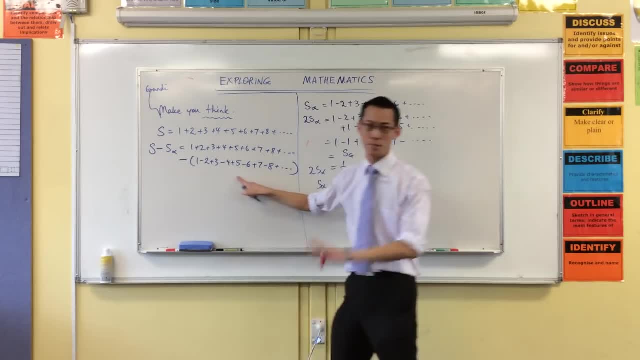 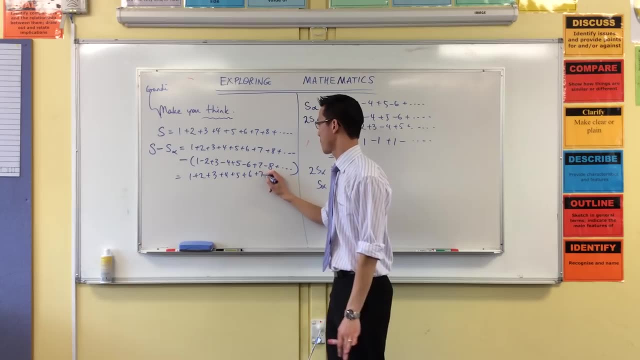 out the front. What does a minus sign do? It flips them all. We saw this before. Okay, No problems. So here's my S, all of the counting numbers there, Okay, And then here's what happens when I subtract the series. 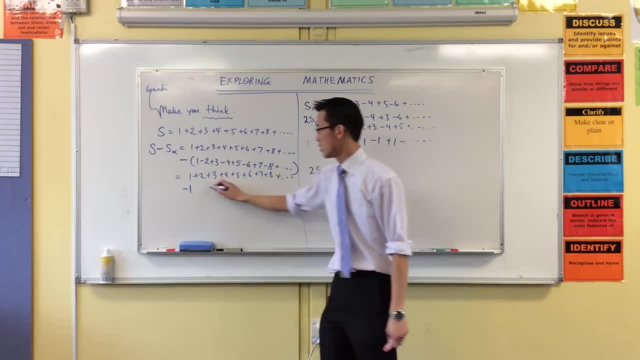 I start with a minus one, Then I get a plus two. What happens to the three? It's minus three Plus four minus five Plus six minus six. Sorry, Is that right? Am I alternating right? Yeah, That looks right. 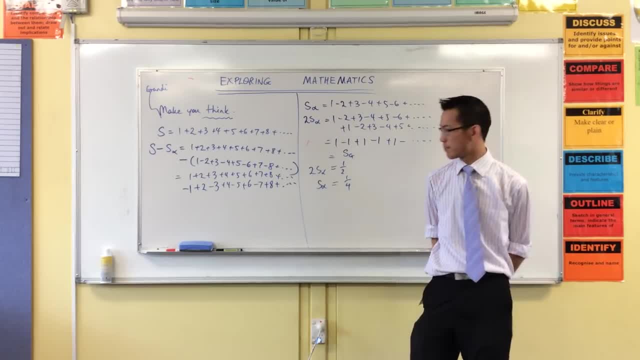 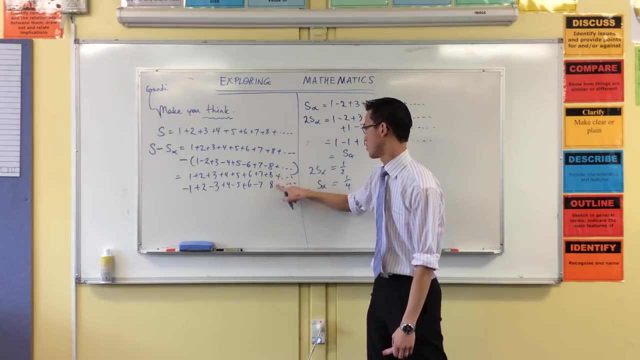 Forever. Okay, Hmm, What's happening? Am I missing a? Oh, sorry, This one, This one, No, after the A: Oh, I see what you mean. That is a plus, isn't it? Yeah, cool. 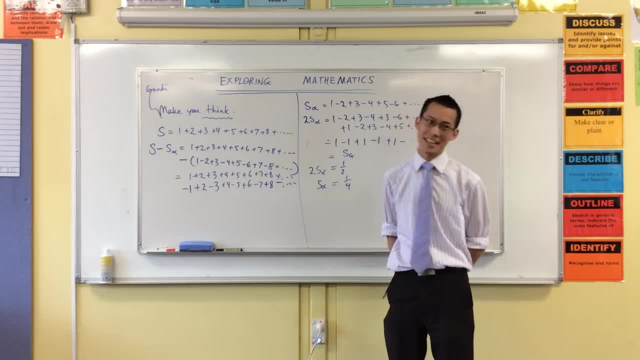 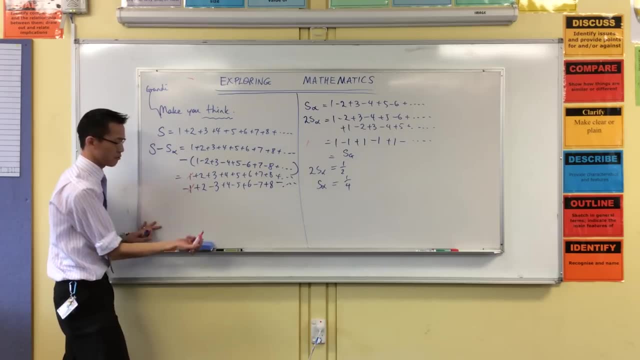 Okay, What happens here? There's some serious cancelling, isn't there Right? How many terms cancel? I've got one. The odd terms cancel, That's exactly right. The ones cancel, So the threes cancel Fives. 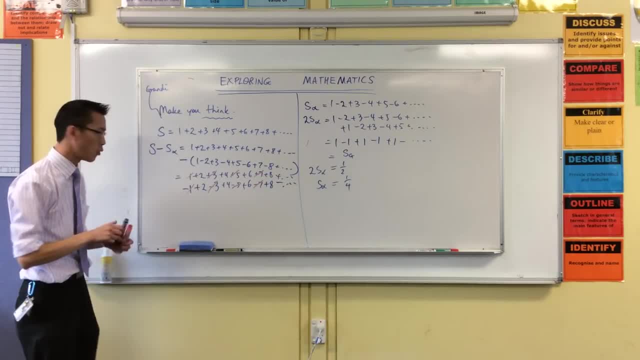 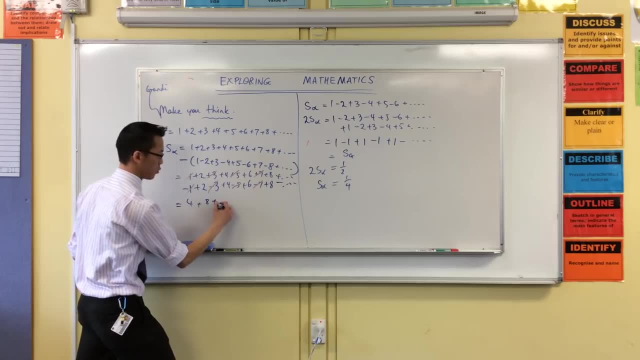 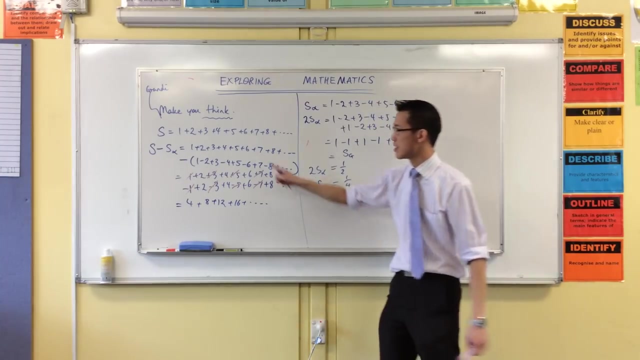 Sevens. So what do you get left with? What do you get left with? Well, by my count, I get a four and then an eight, and then a twelve. What are these? This is this guy, but four times bigger. Every term is four times bigger, is it not? 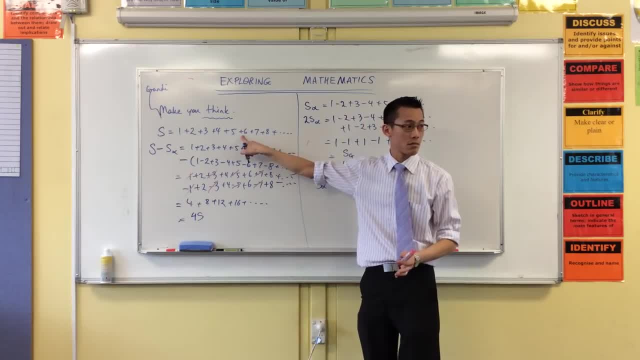 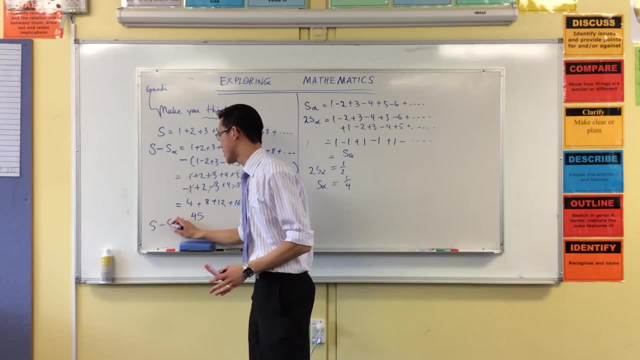 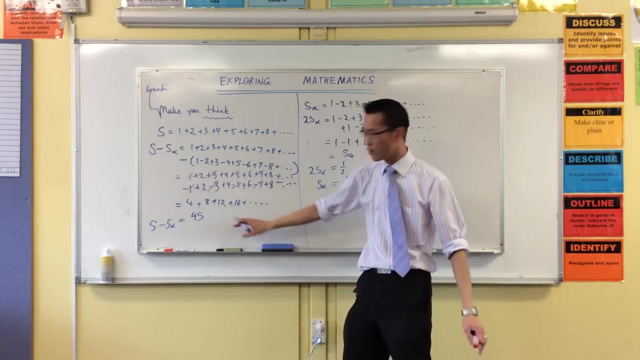 So this is four times this. Oh, Isn't it? Hold on, Hold on. We subtracted something and it got bigger. What does that mean? I'll show you what it means. Look, look, look. We know what S alpha. 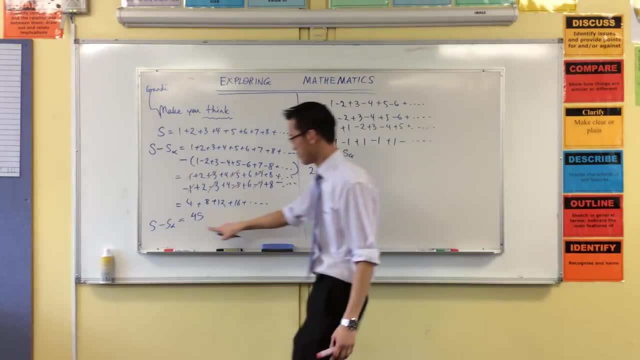 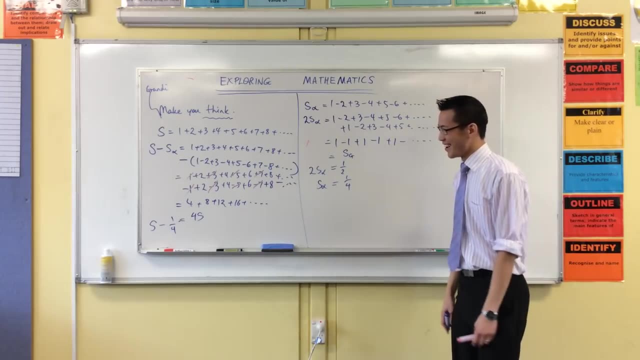 is this sum: It's a quarter, It's a quarter, So I'm just going to take that out. Is that alright? You happy with that? How do I get this? I want to know what this thing is equal to. 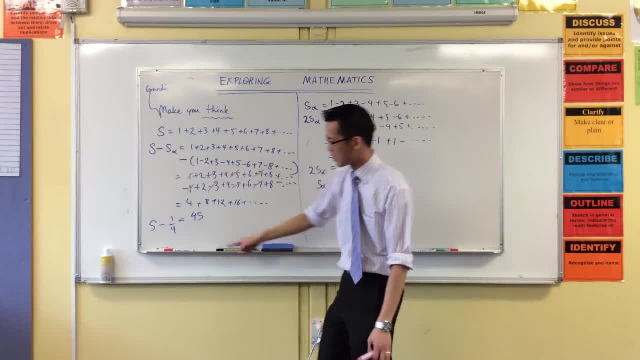 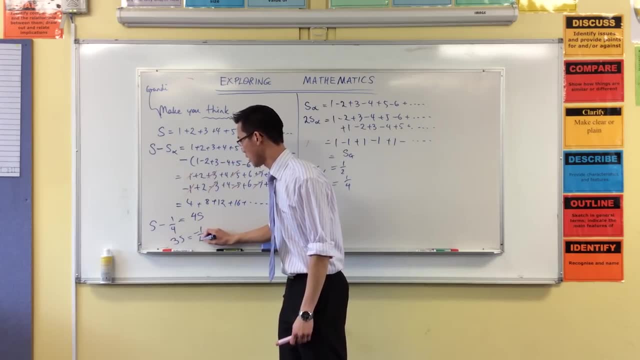 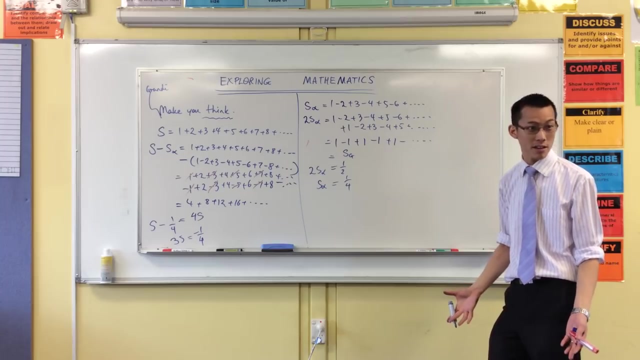 Right. Okay, How do I rearrange this thing? Looks to me like I should take one S over here, Subtract S from both sides. Looks to me like I get three S equals negative a quarter. So I should divide by three, Right, Right? 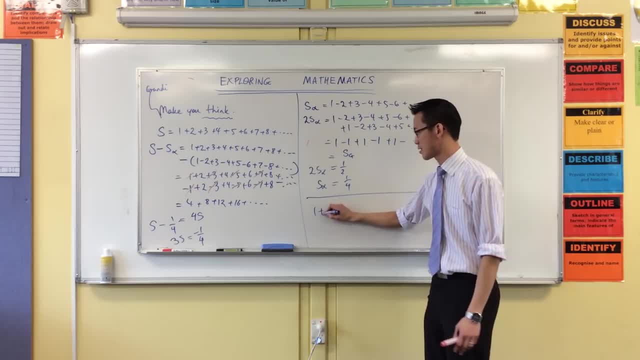 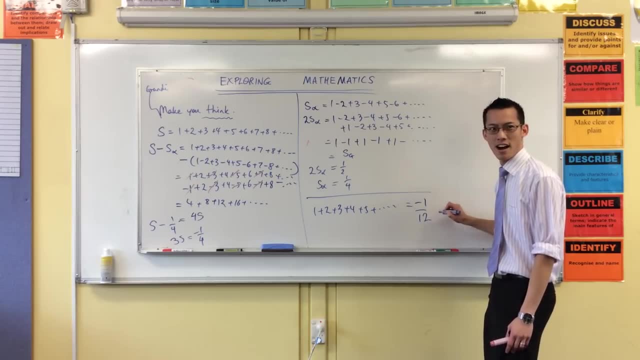 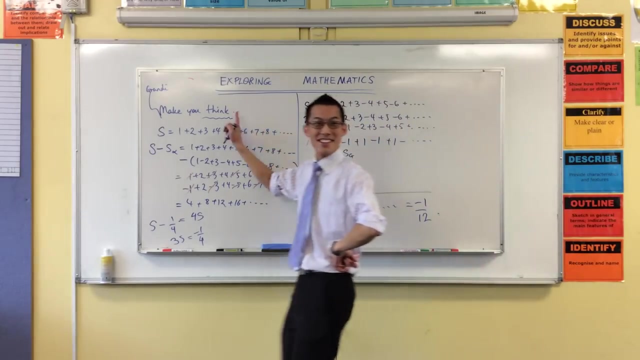 If I divide by three, I'll get back here. I'll get back to this boring infinity series, Right? Oh wait, He's not infinity After all. Have I made you think yet Now you can go off and search. 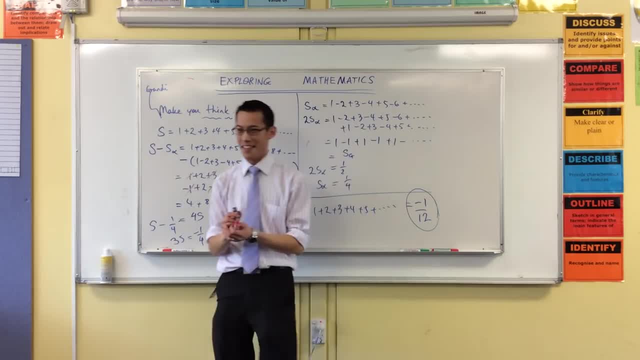 In fact go and look on. if you're really that unable to go past the first couple of results on Google, Go and look for the Wikipedia argument called it's named negative one over twelve, And you will find this proof and quite a bit of discussion. It's a controversial. 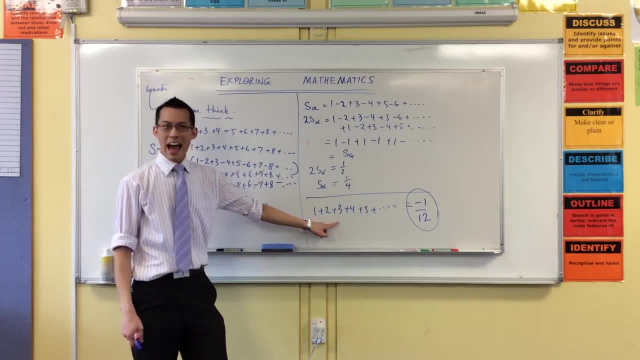 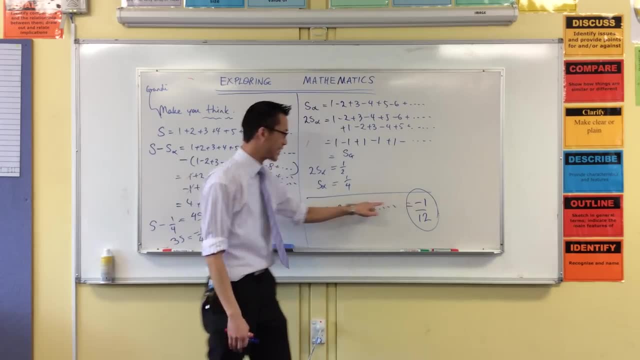 result? Of course it's a controversial result. How can you add up a whole bunch of positive numbers, not only get a negative, but get a negative fraction? You're all fired. You clearly didn't pick up. I must have made a mistake somewhere. 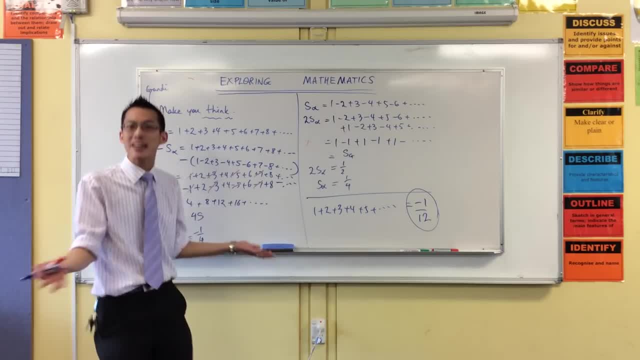 Right, Right. Well, you can go and scrutinise. Like I said, I did not make up this proof. It's a well-known thing. The question is: what does it all mean? It's a well-known thing. The question is: what does it all mean?